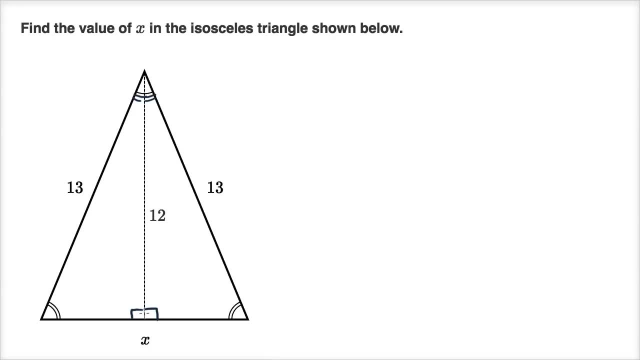 and you have a side between them that is the same. this altitude of length, 12 is on both triangles. we know that both of these triangles are congruent, So they're both gonna have 13,. they're gonna have one side, that's 13,. 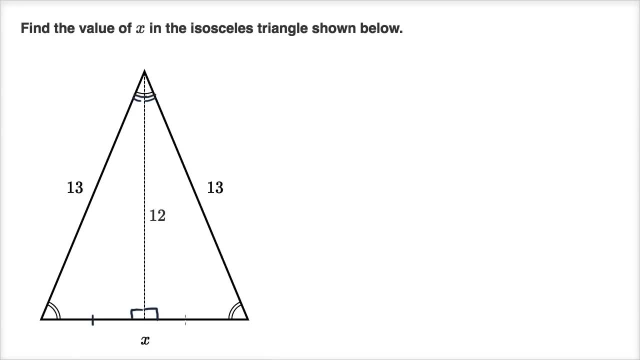 one side, that is 12, and so this and this side are going to be the same. So this is going to be x over two, and this is going to be x over two, And so now we can use that information and the Pythagorean theorem to solve for x. 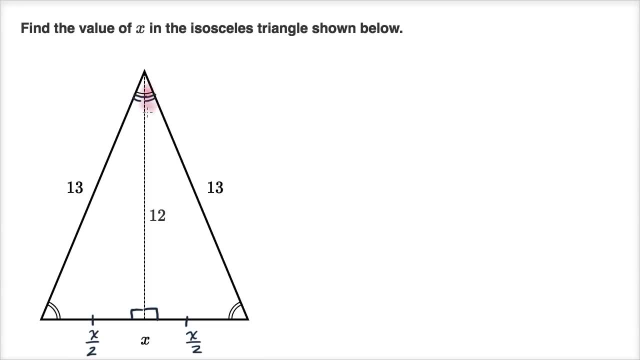 Let's use the Pythagorean theorem on this right triangle. on the right-hand side, We can say that x over two squared, that's the base. right over here, this side, right over here, we could write that x over two squared plus the other side, plus 12 squared. 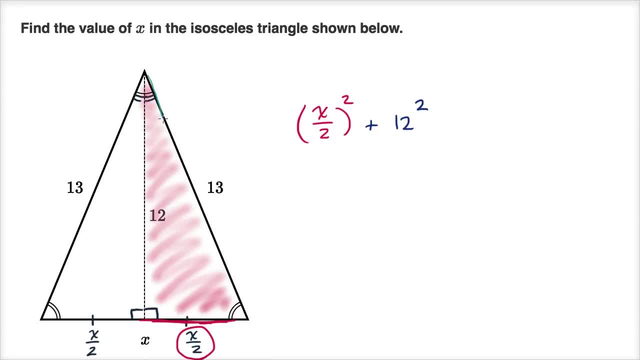 is going to be equal to our hypotenuse squared is going to be equal to 13 squared. This is just the Pythagorean theorem now, And so we can simplify: This is going to be x. we do that same color. 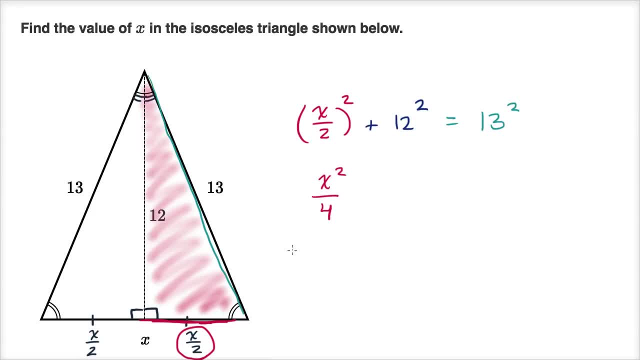 this is going to be x squared over four. that's just x squared over two, squared plus 144,. 144 is equal to 13. squared is 169.. Now I can subtract 144 from both sides. I'm gonna try to solve for x. 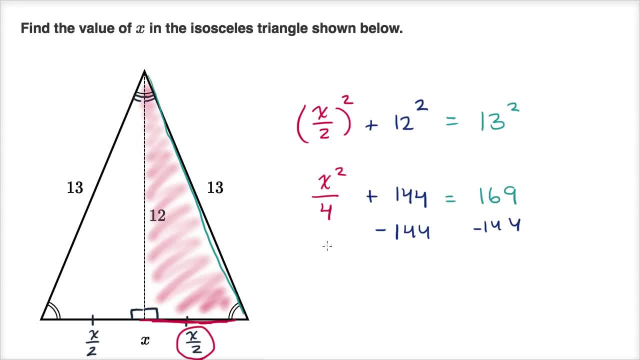 that's the whole goal here. So subtracting 144 from both sides, and what do we get? On the left-hand side, we have x squared over. four is equal to 169 minus 144.. Let's see: 69 minus 44 is 25.. 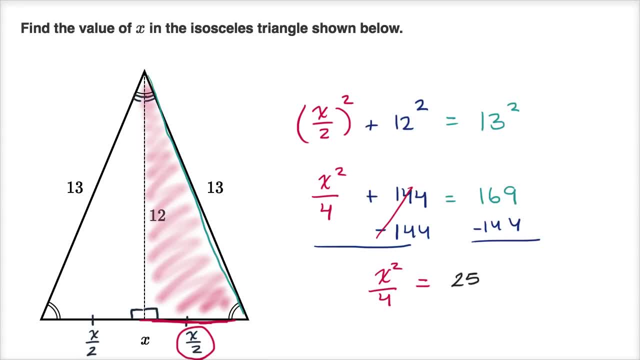 So this is going to be equal to 25.. We can multiply both sides by four to isolate the x squared, And so we get: x squared is equal to 25 times four is equal to 100.. Now if we were just looking at this purely mathematically, 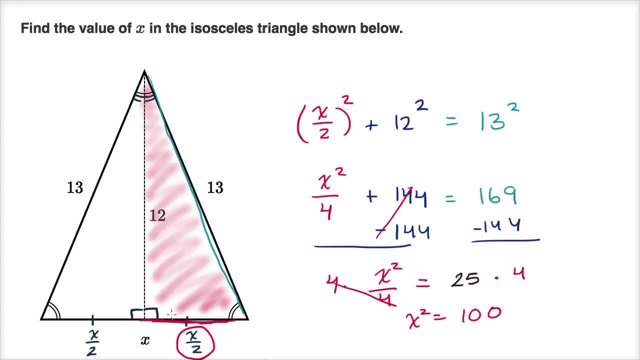 you'd say, oh, x could be positive or negative 10.. But since we're dealing with distances, we know that we want the positive value of it. So x is equal to the principal root of 100,, which is equal to positive 10..